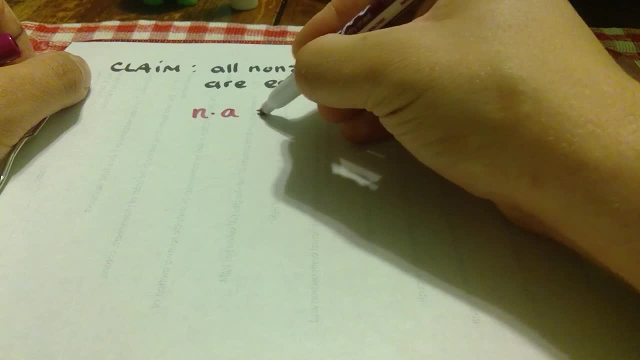 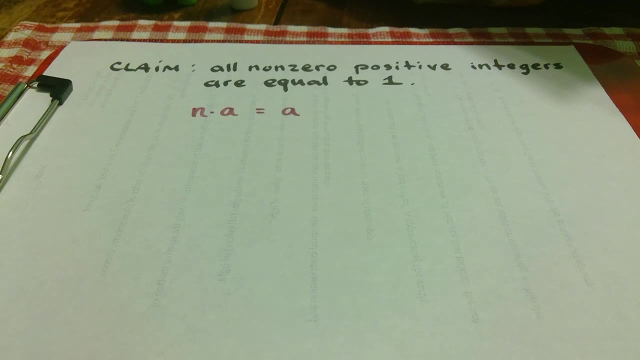 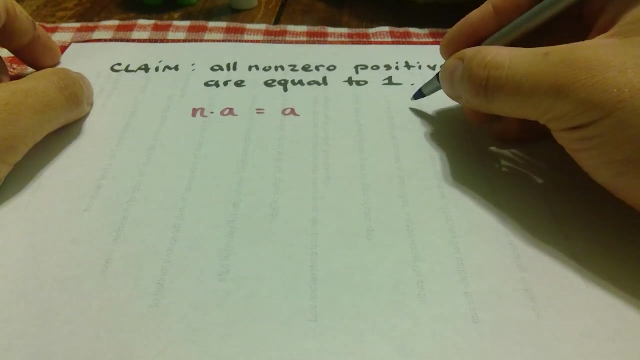 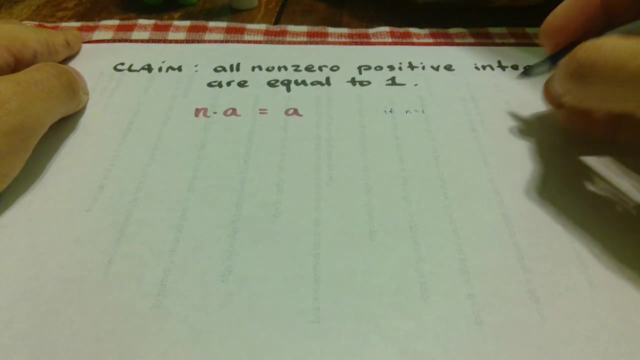 to any nonzero number, a, we end up getting that same number back. This is a basic fact of multiplication. Now, why is this the case? Well, let's go ahead and write down a few cases. So, first of all, if n is equal to 1, then we have 1 times a is equal to a. Pretty pretty good. So if n is equal to 1, then we have 1 times a is equal to a Pretty pretty good. So if n is equal to 1, then we have 1 times a is equal to a Pretty pretty good. 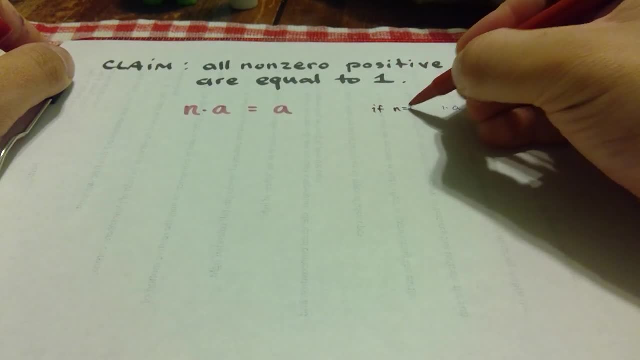 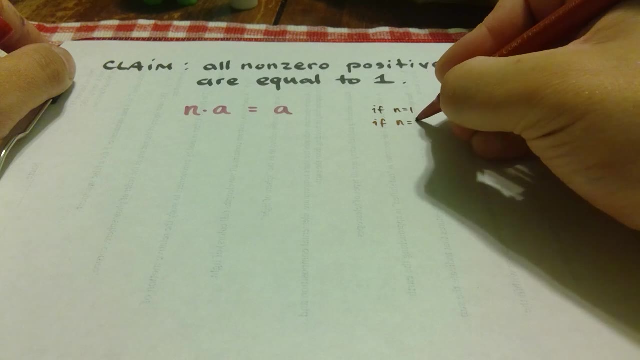 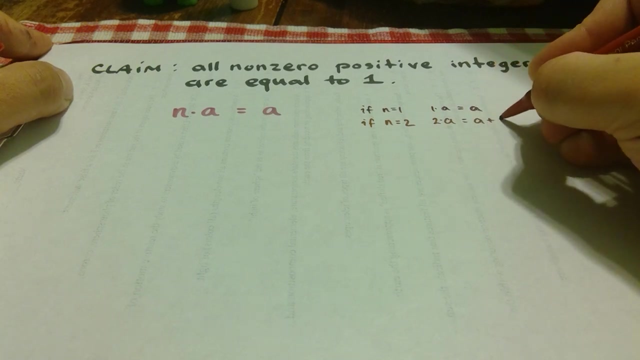 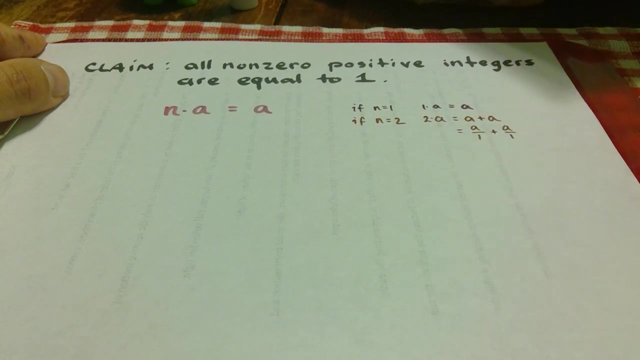 Pretty simple, right? If n is equal to 1, then we have 1 times a, which is equal to a. What about if n is equal to 2?? Well, if n is equal to 2, then we have what: 2 times a is equal to a, plus a, which is equal to a over 1, plus a over 1, and we have 2 fractions. How do we add fractions together? Of course, we need to add the numerator. 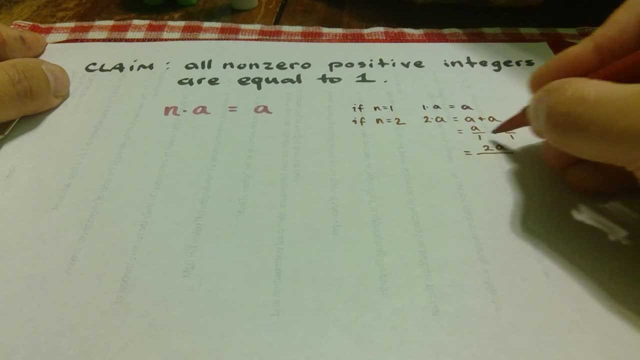 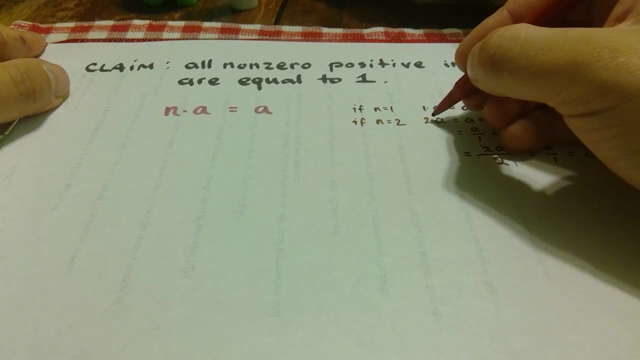 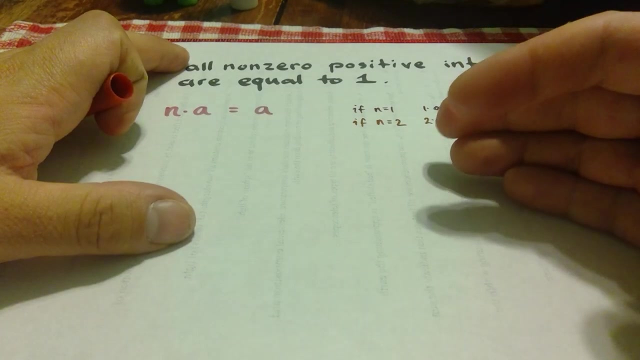 together. So we have 2a over, and then we add the denominators 2a over 2. And then we can cancel out the 2s. Of course this is going to turn into 1. And we end up with a over 1, which is equal to a. So 2a is equal to 2 times a is equal to a. Now this will be true for the nth case as well. Let's go ahead and do that. Suppose we take n and we multiply it by 2.. 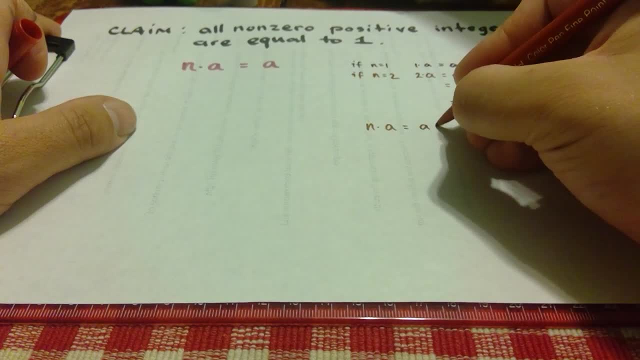 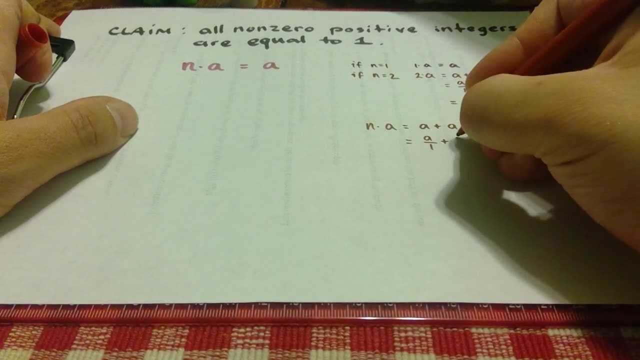 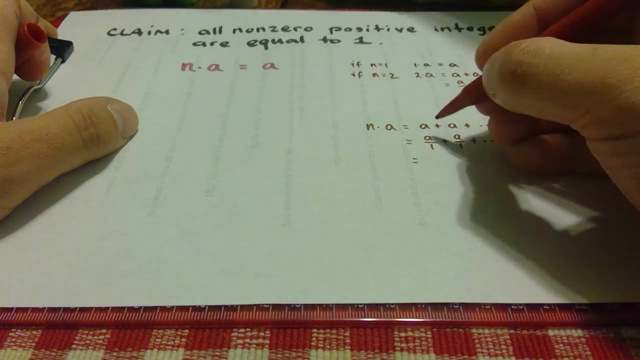 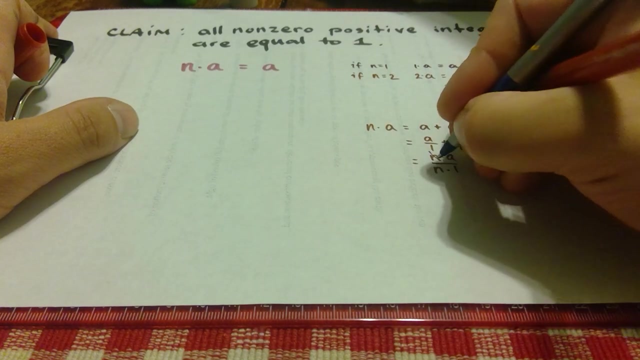 And we multiply it by a. What happens? This is the same as a plus a plus dot, dot dot plus a, which of course is a over 1 plus a over 1 plus dot dot dot plus a over 1.. Again, we're adding a bunch of fractions. here We have to add the numerators and denominators, So we're going to have n times a over n times 1.. Cancel out your n's. You end up with a over 1, which is equal to a. So basically, 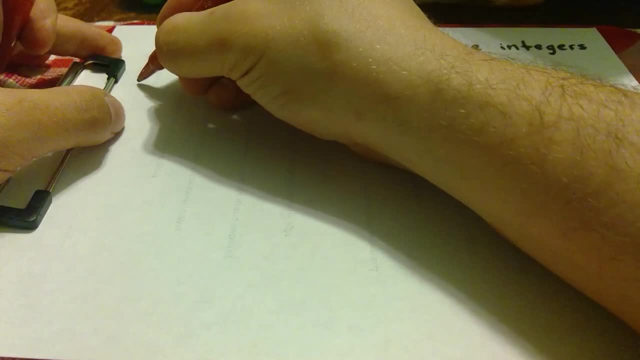 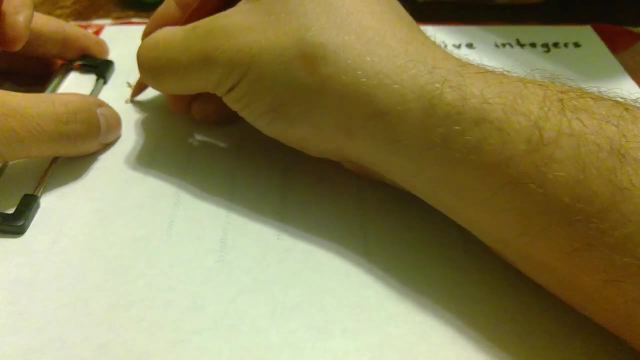 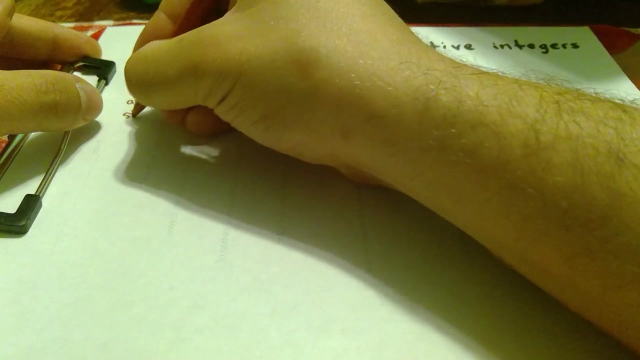 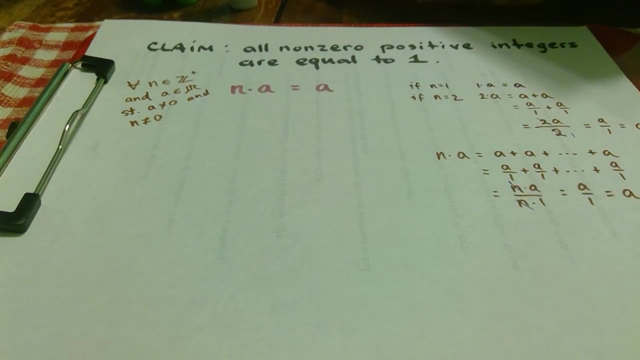 for all, n in the positive integers and a in the real numbers, such that a is not equal to 0 and n is not equal to 0.. We have this identity. We have this identity. So this will be the starting point of our proof. 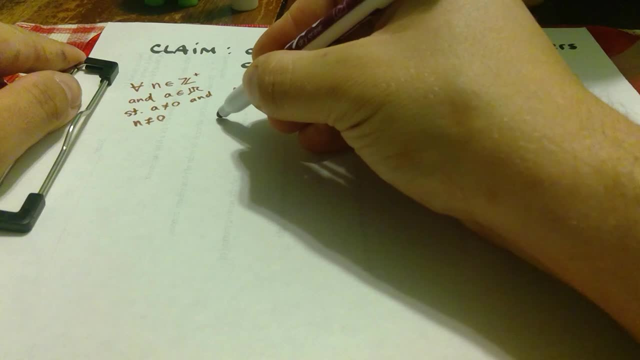 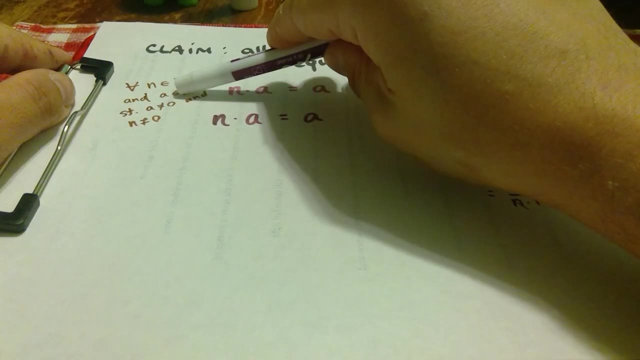 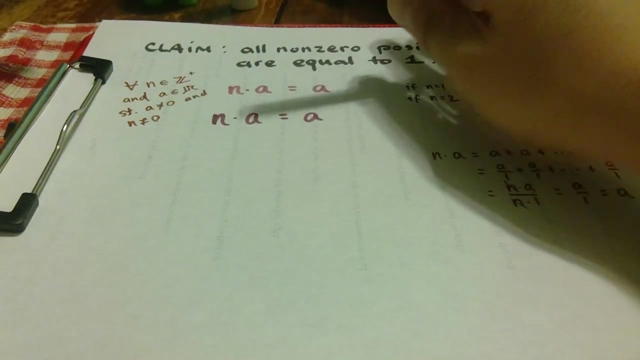 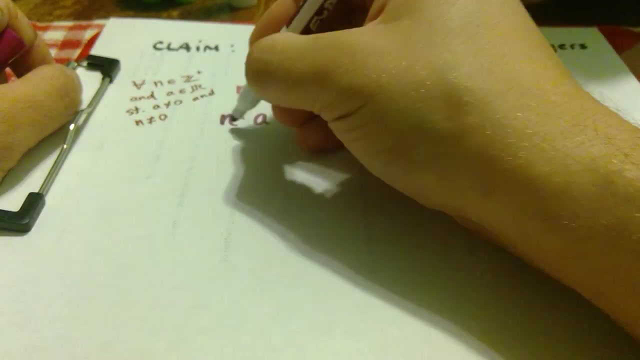 What we need to do is simply observe that a is a real number that's different from 0. Because a is different from 0, we're able to divide by it, So we can use the cancellation property of equality. So, essentially, which amounts to dividing both sides by a number. So we end up dividing both sides And we end up dividing the. 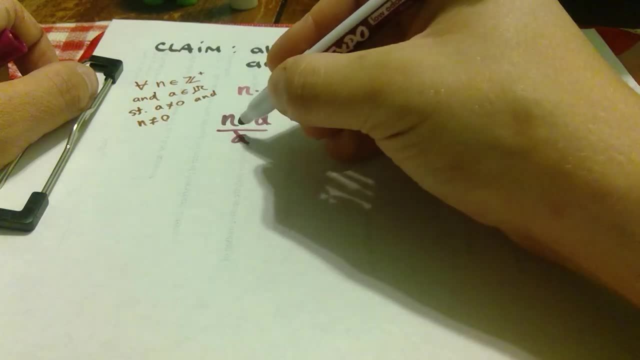 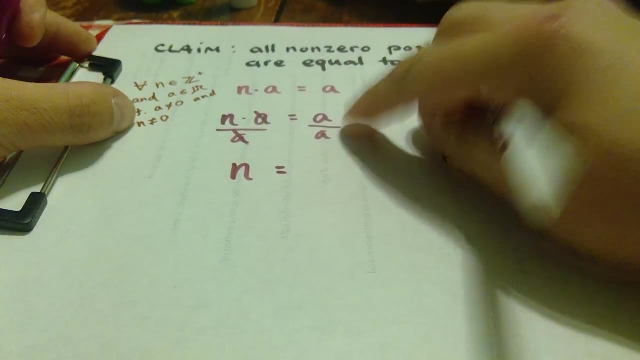 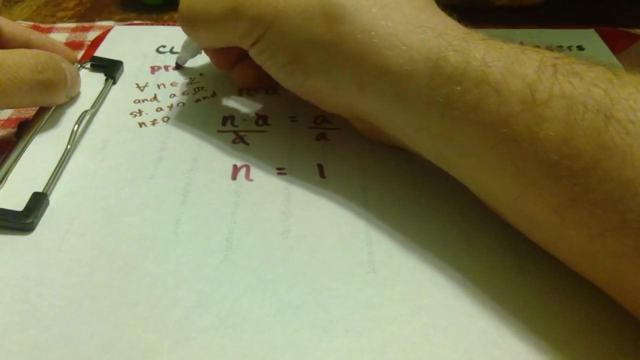 of this equation by a. and what happens here? well, here we have n times a over a, which is 1. n times 1 is n, and on the other side we have a over a, which, of course, is just 1. so the proof is pretty straightforward. you start with the fact: 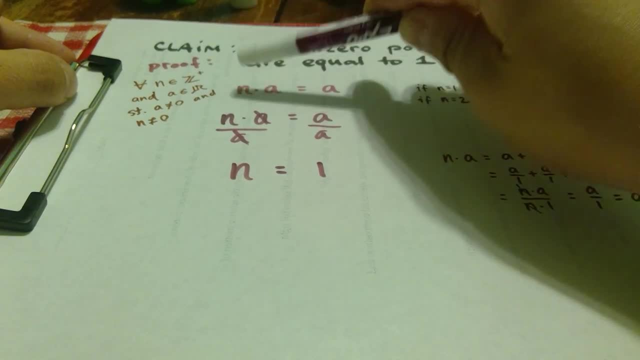 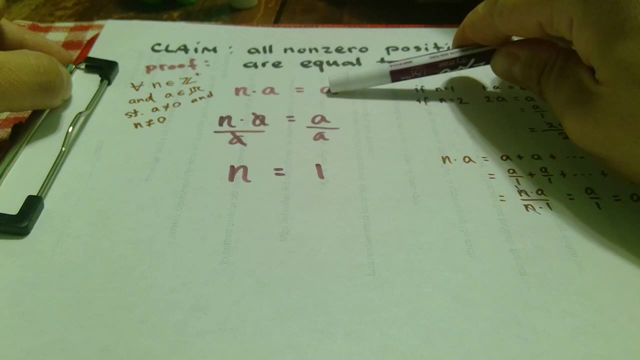 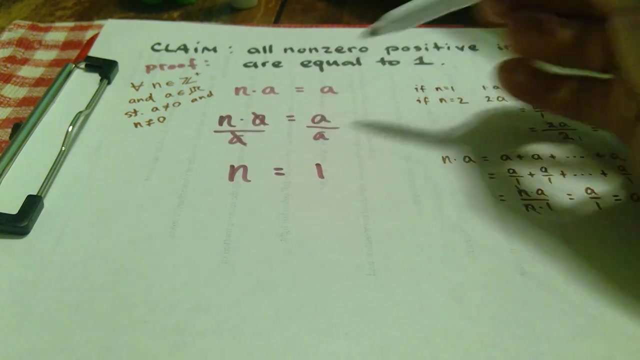 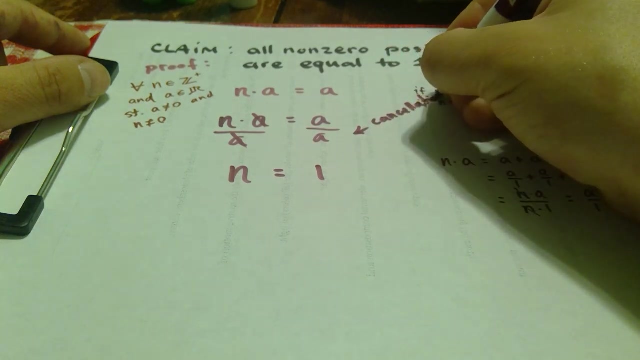 that when you multiply any positive nonzero integer by any nonzero real number, you get that same nonzero real number back. okay now, precisely because a is a nonzero real number, we can divide both sides by it, using the cancellation property right. this is cancellation right here, and that gives us our result. 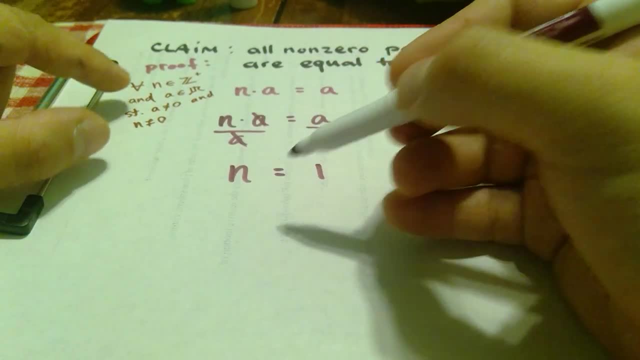 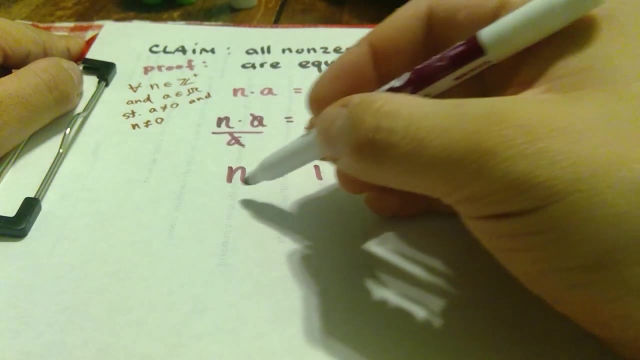 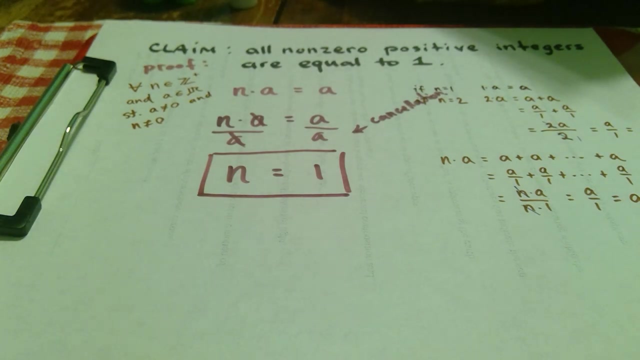 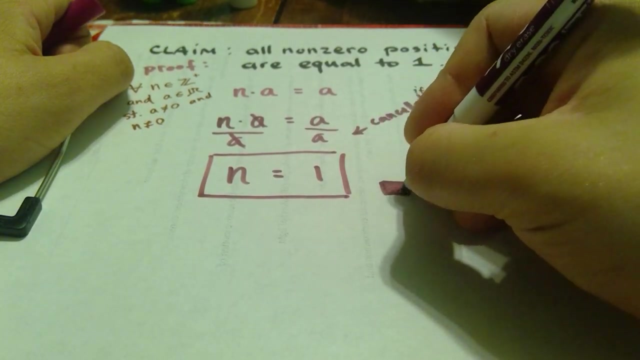 n is equal to 1, and this is what this is for all n in the positive integers, such that n is not equal to 0. so we have just proven that every nonzero positive integer is equal to the number 1. and what do we do? draw a little square or a little rectangle and shade it in.